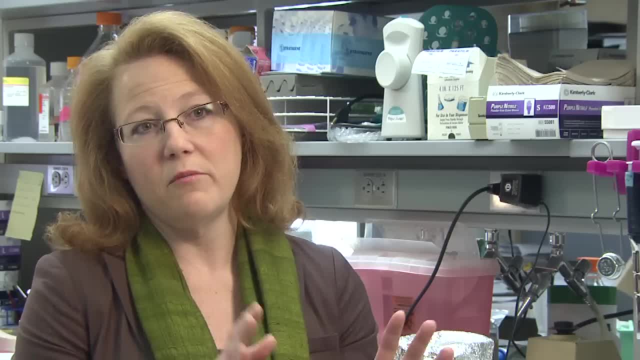 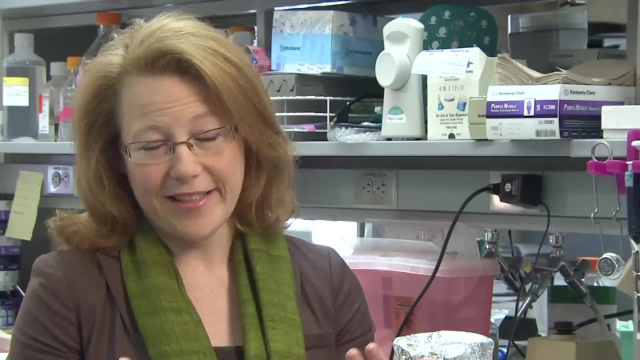 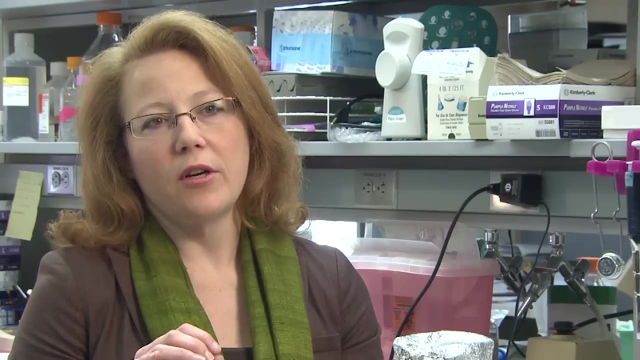 we induced either a positive or a negative mood state and then observed how mood influenced their subsequent smoking behavior. And what we found from that first study was that women, as we expected- it's always nice when they work out- is that women when we induced a negative mood? 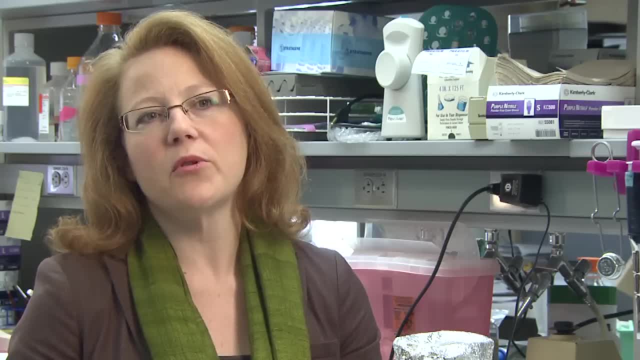 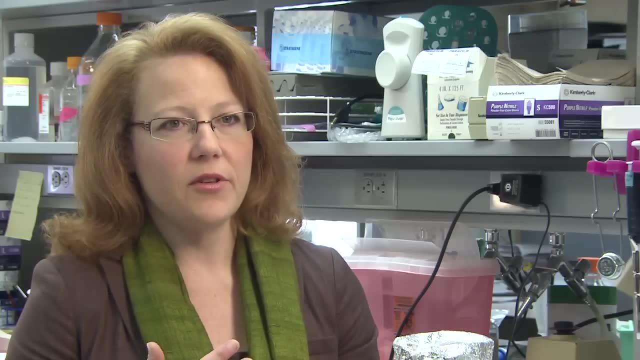 were more likely to smoke more quickly and they also smoked more intensely And that means they inhaled more deeply off their cigarettes. they took more puffs off their cigarettes. they had shorter intervals of time in between their puffs, so they just smoked the cigarettes more intensely. 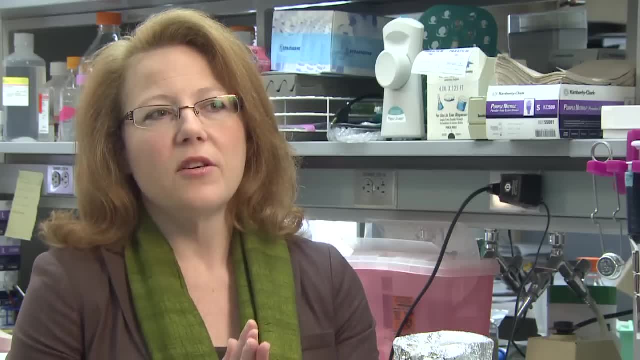 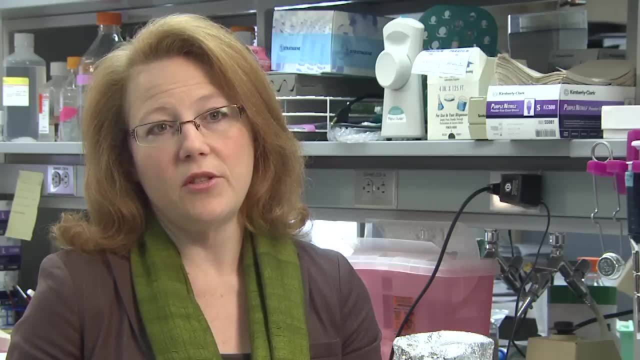 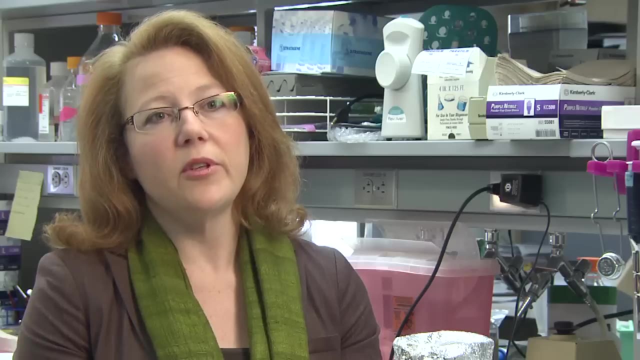 and also smoked more cigarettes overall. So from this initial study, we've now been able to secure two additional grants from the National Institutes on Health to develop a laboratory model to look at how negative mood and stress influences relapse. What we find within this laboratory model is that stress, of course, 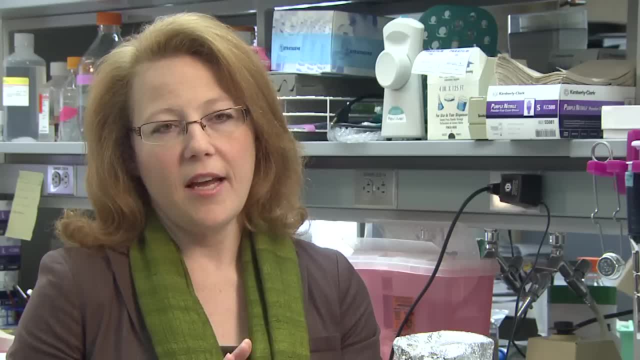 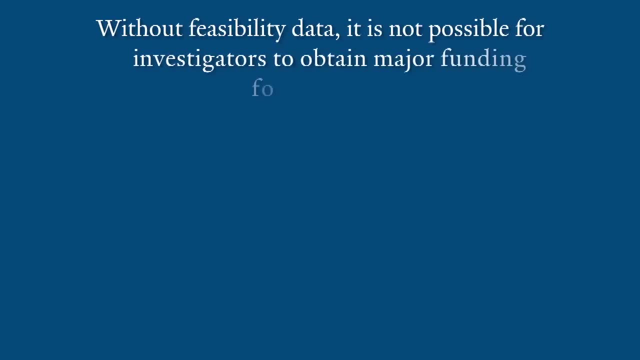 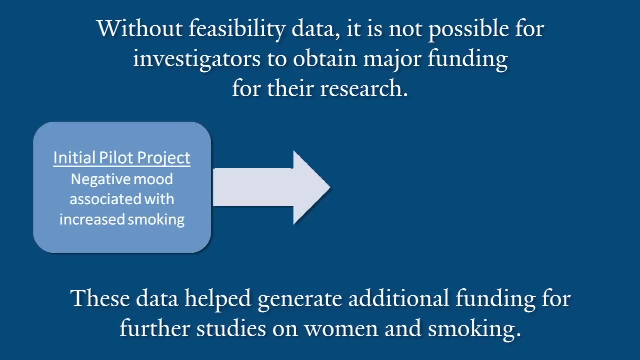 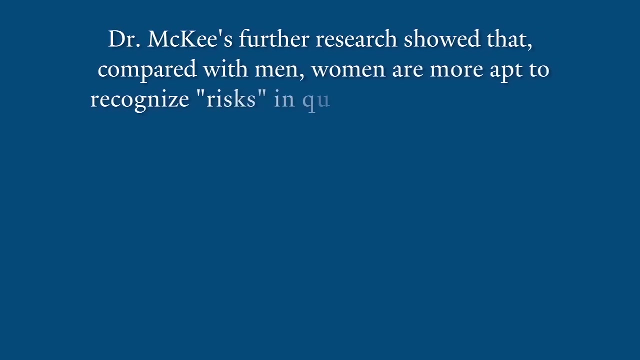 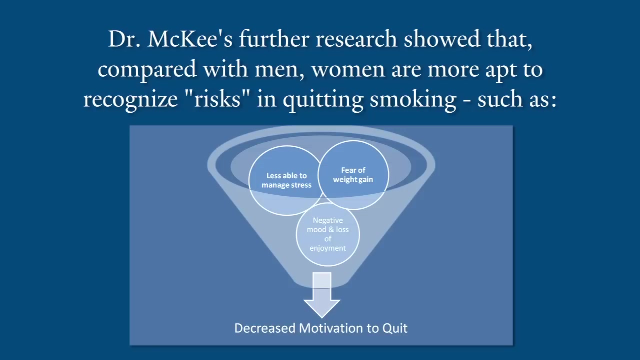 decreases their ability to resist smoking and it increases the amount of subsequent smoking. But if you're not able to resist smoking, you're not able to resist smoking. So the research focuses on the benefits of quitting. So, of course, you're going to improve your health. 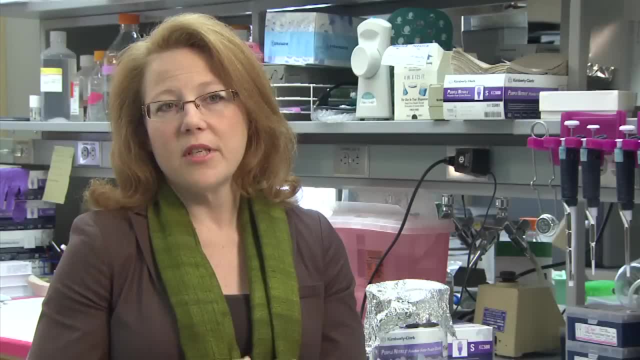 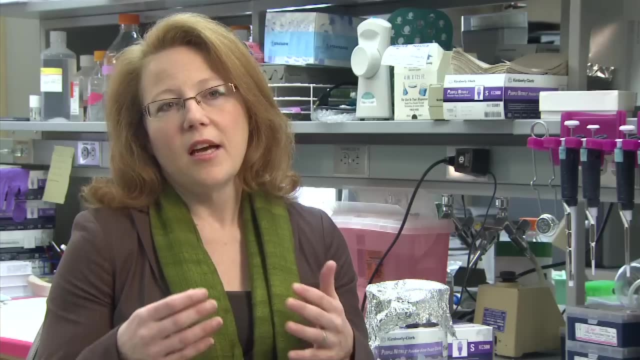 you're going to save money, et cetera. But women acknowledge and experience significant risks associated with quitting. So they say: if I quit smoking I'm going to be less able to manage my stress, I'm going to gain weight. 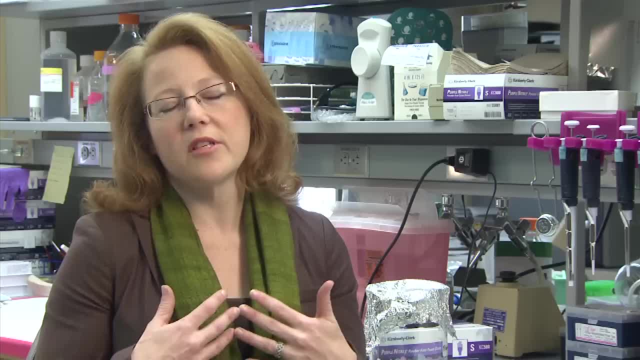 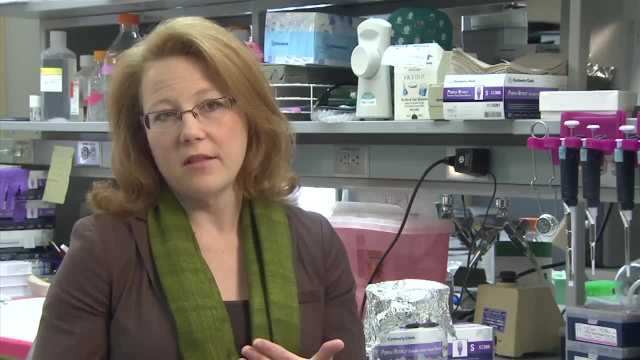 I'm going to lose this ability to handle myself. I'm going to lose the ability to get to work. I'm going to lose the ability to get to work. I'm going to lose the ability to get to work. I'm going to lose a significant source of enjoyment out of my life. 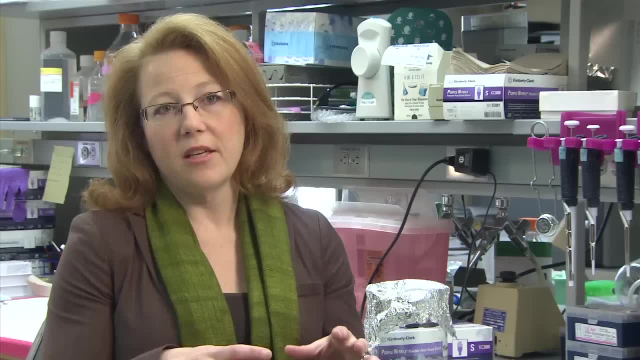 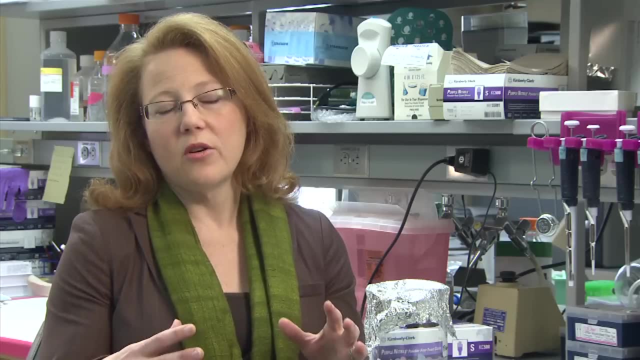 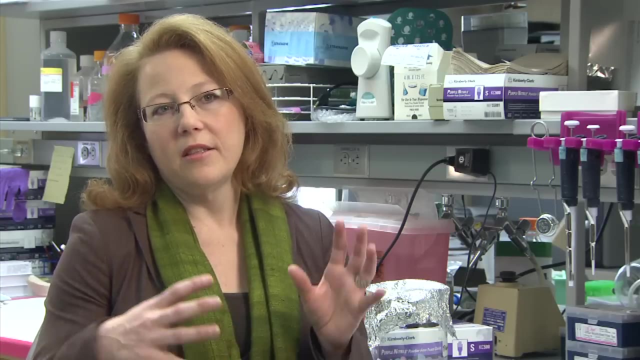 So we've shown that these risks are associated with lower motivation to quit smoking and are also associated, and so if women do try to quit, these risks are also associated with less success in quitting smoking. So we've been targeting these risks in terms of treatment development. 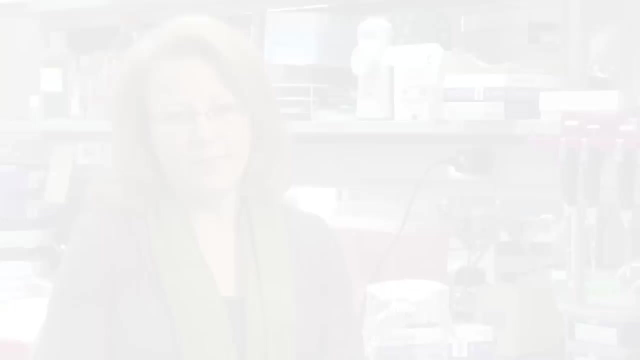 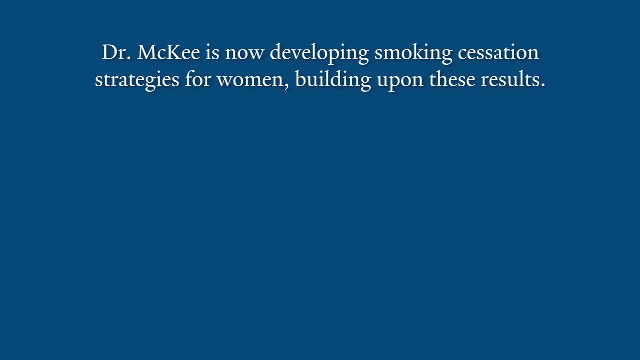 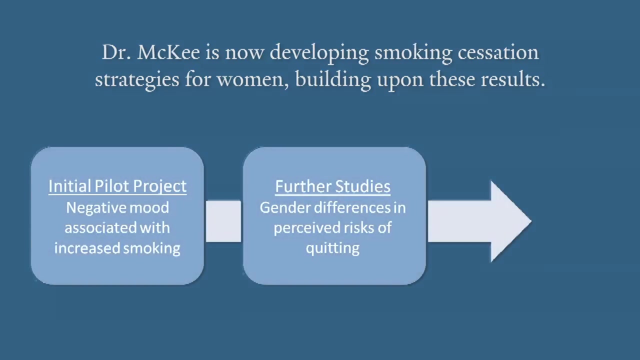 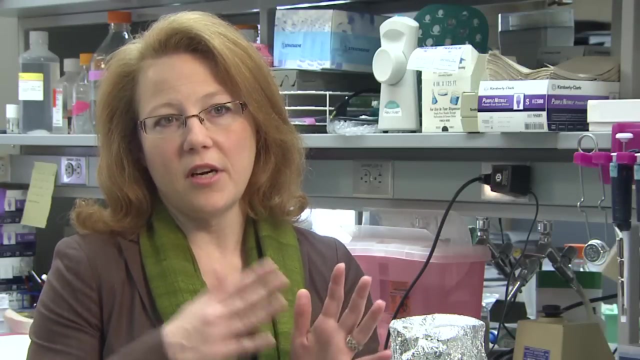 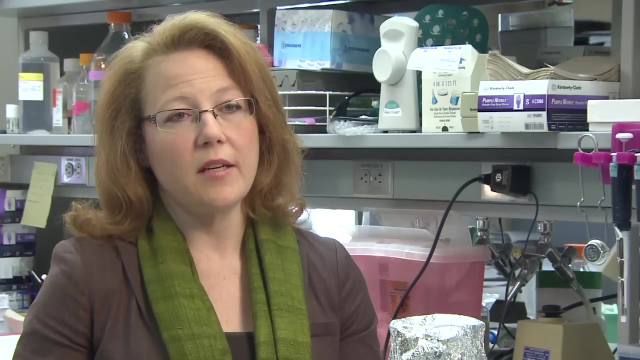 and trying to develop more effective treatments for women. So now that we've developed this laboratory model, we're now using it to screen medications that are designed to target the effect of stress on smoking behavior. So this is a relatively novel strategy for smoking cessation medications. 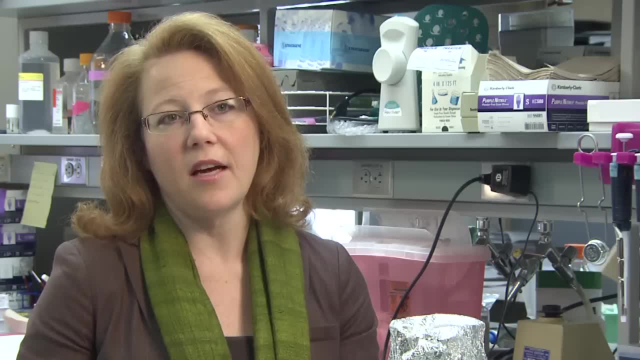 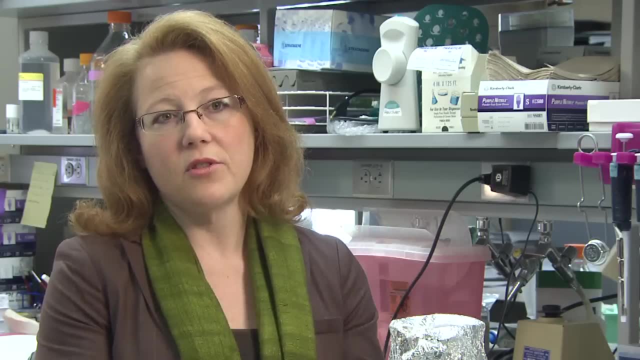 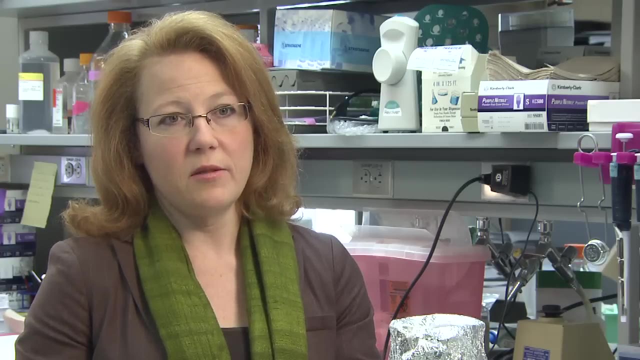 because, up to this point, medications have been designed to target either nicotine reinforcement or withdrawal symptoms and not target the effect of stress on smoking behavior, And we know from our prior work that stress is a primary reason why smokers continue smoking, and this is particularly true for women. 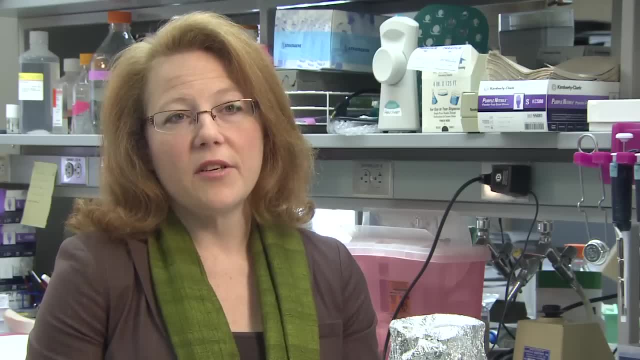 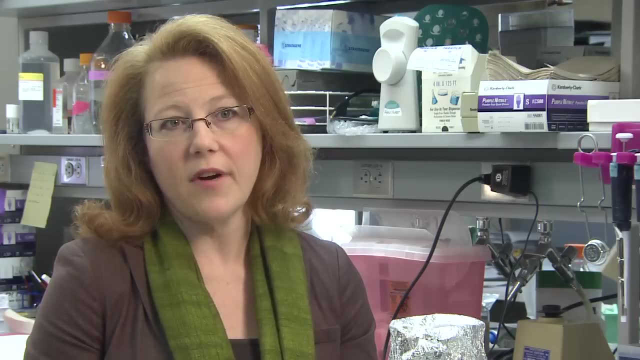 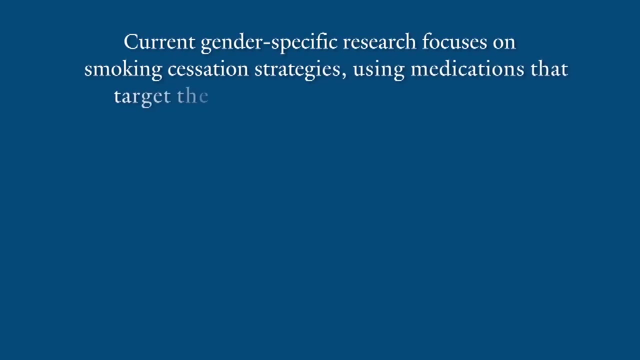 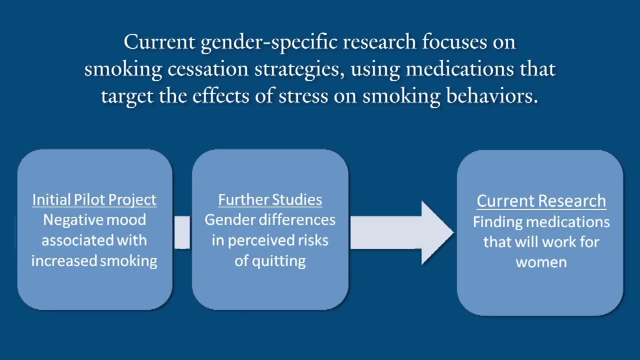 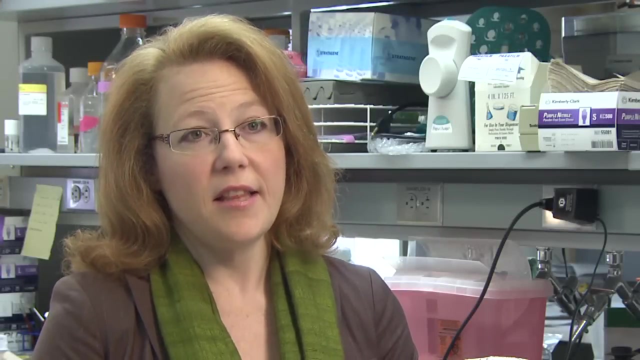 and then why they relapse back to smoking. We have been researching how various medications target the effect of stress on smoking behavior, and I would say that these are our most important findings to date. We've identified a class of medications that does reduce the effect of stress on smoking behavior, so we're quite excited. 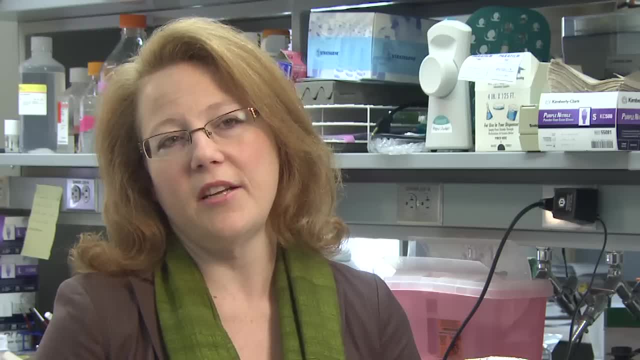 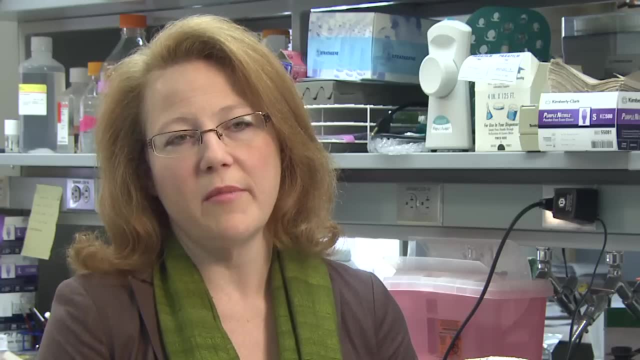 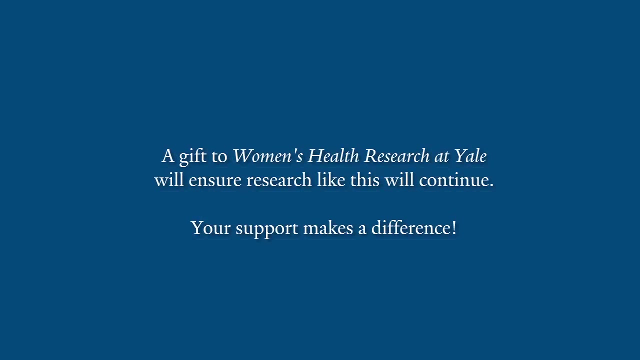 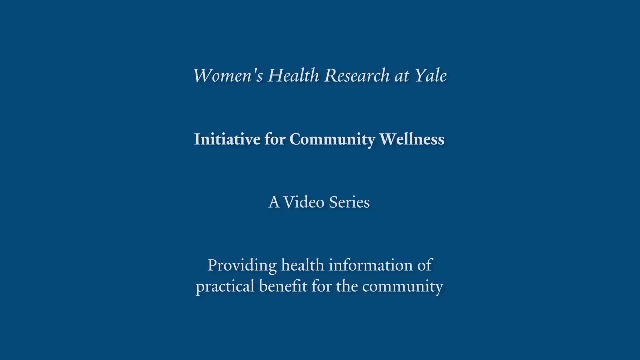 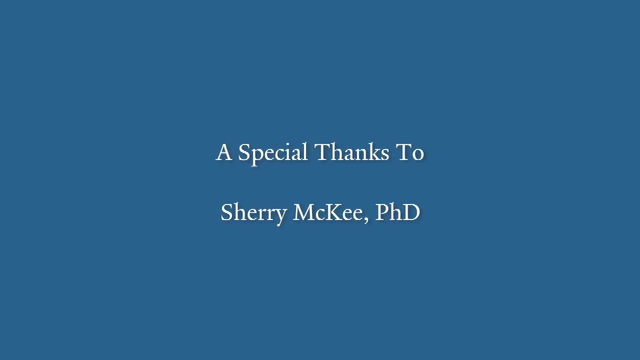 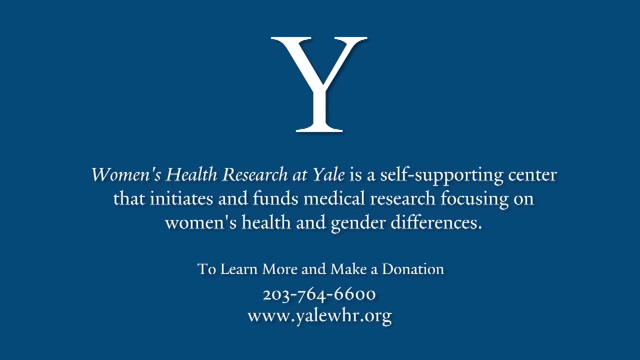